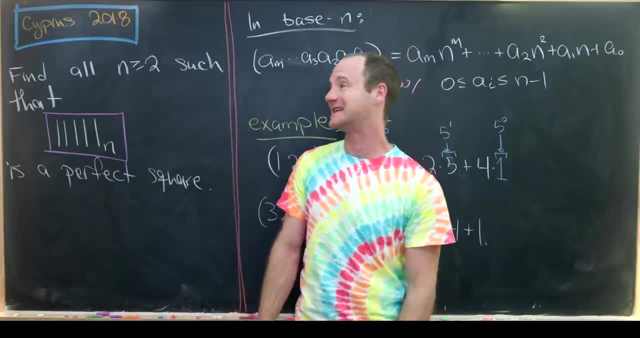 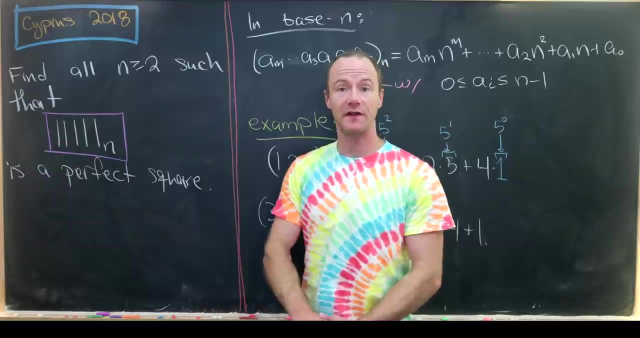 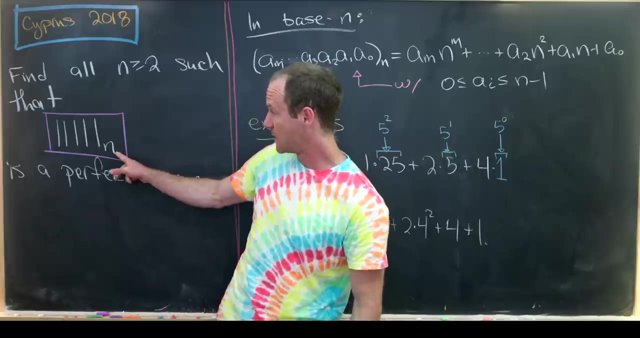 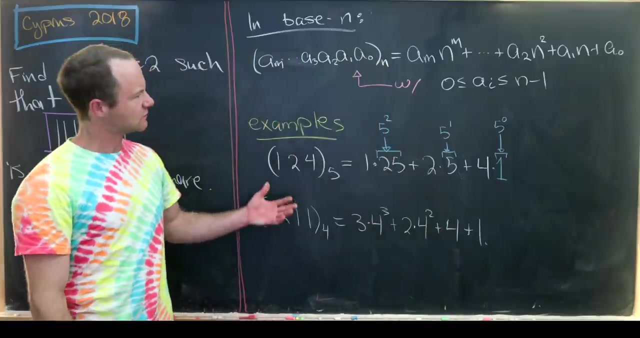 Here I've got this nice problem that's from the 2018 Cyprus National Math Olympiad, So let's see what it says. Our goal is to find all natural numbers that are bigger than or equal to two, such that in base n, the number 1, 1, 1, 1, 1,- that's, five ones- is a perfect square. So let's just 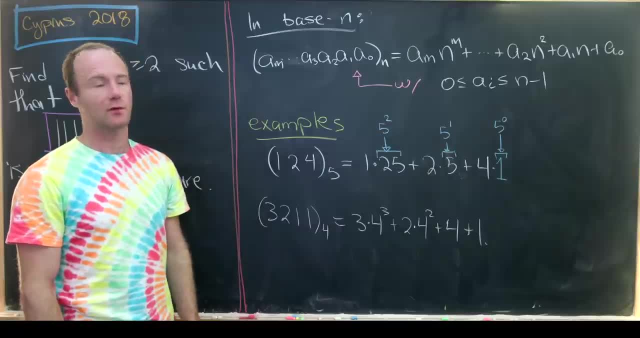 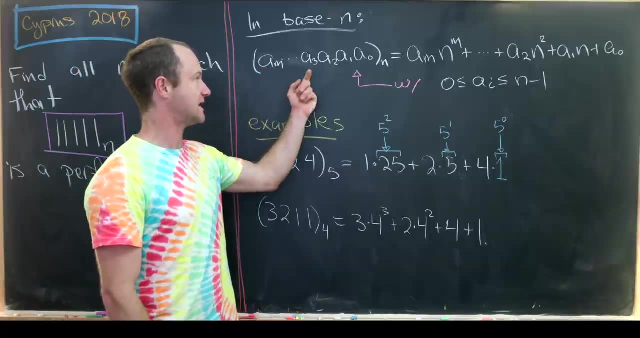 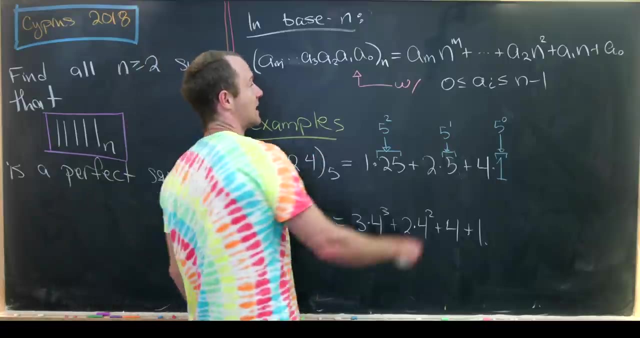 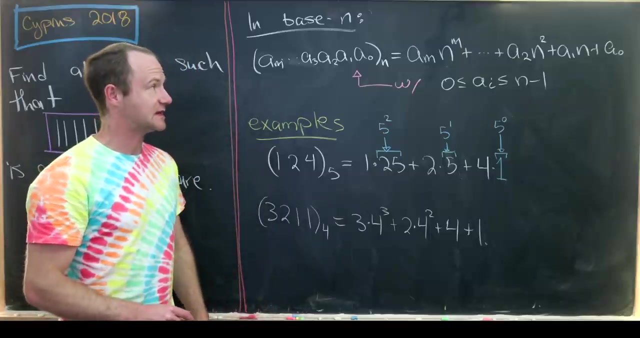 recall what it means to write a number in base n expression before we get started. So a number written in base n that has digits: a m, a m minus 1, all the way down to a 3, 2, 1, 0 base n. so that's what I have here is the sum: a sub m n to the m plus a sub m minus 1 n n to the. 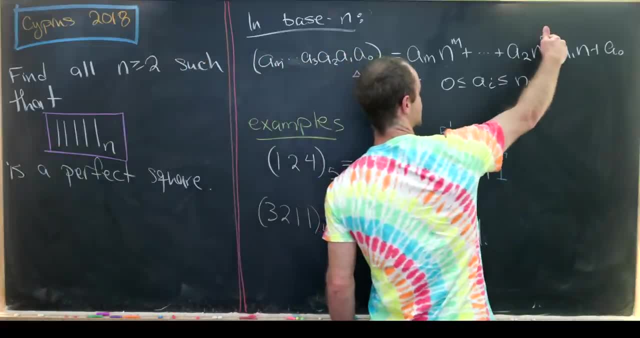 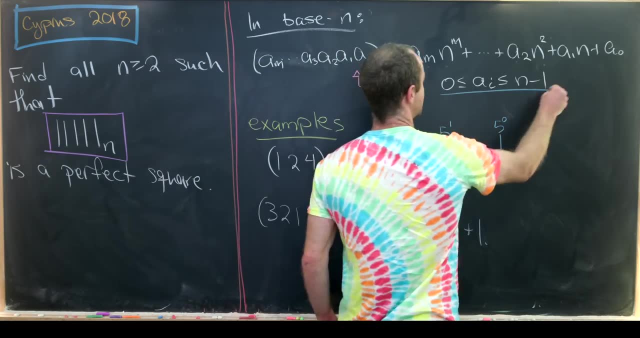 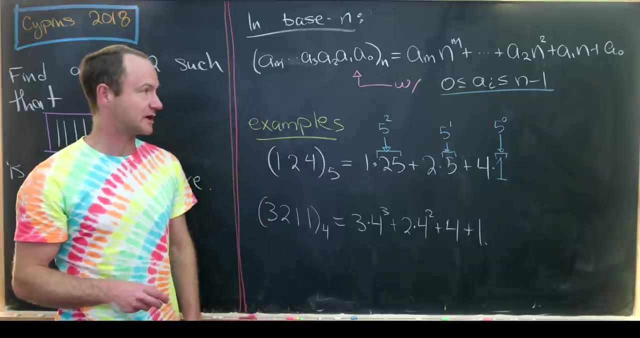 m minus 1 plus all the way down to a sub 2 n, squared a sub 1 n plus a sub 0. And generally you take a i, a, i a i to be between 0 and n minus 1.. There's actually a nice Putnam problem that asks you to look at. 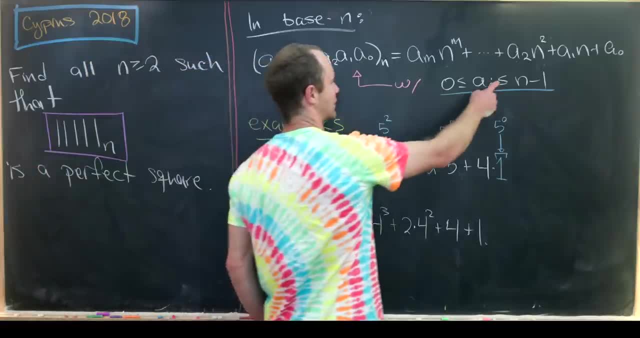 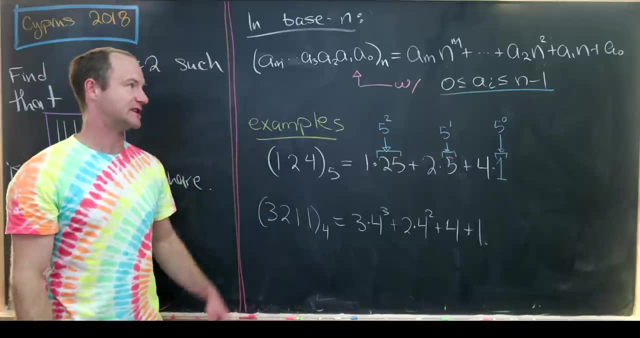 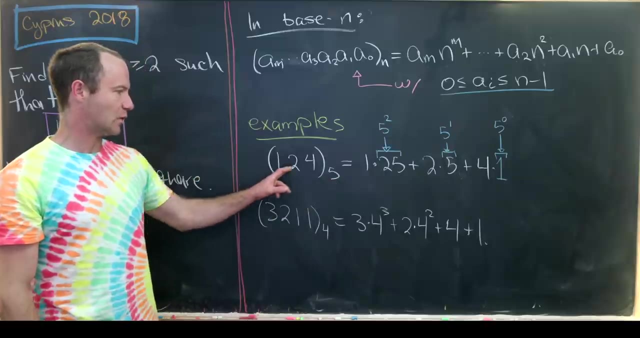 base 10 over representations where you allow this a i to be equal to 10.. But apart from that problem, you always take those digits to be between 0 and 1 less than the base. So here are a couple of examples. So in base 5, the number 1, 2, 4 is 1 times 25 plus 2 times 5 plus 1 times. 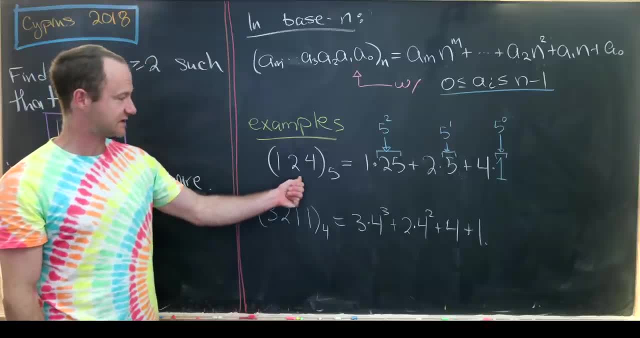 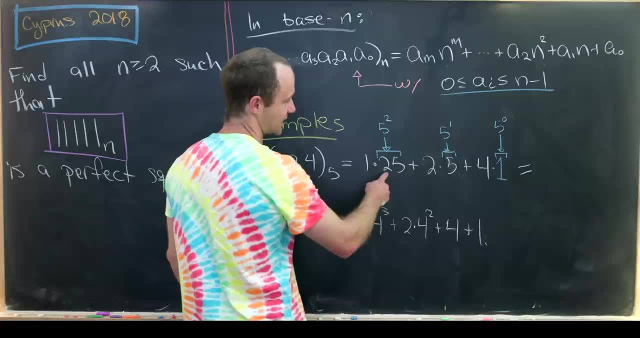 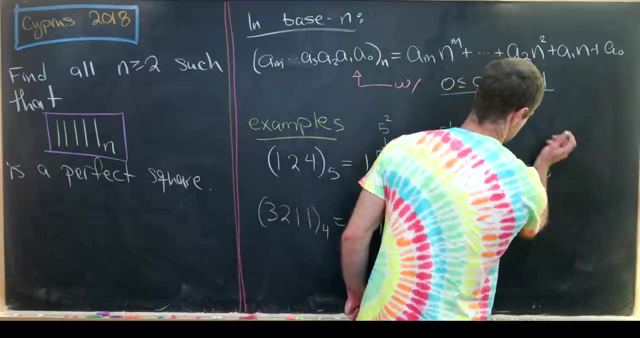 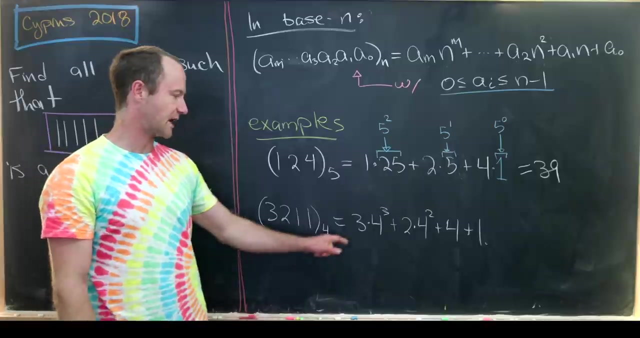 3 times 4 plus 4.. This is the 5 squared digit. This is the 5 to the first digit. This is the 5 to the zero digit. So, written in base 10, what do we have here? Well, that's going to be 25 plus 10.. So that 35 plus 4 is is 39. And then, in base four, the number 3, 2, 1, 1, that will be. 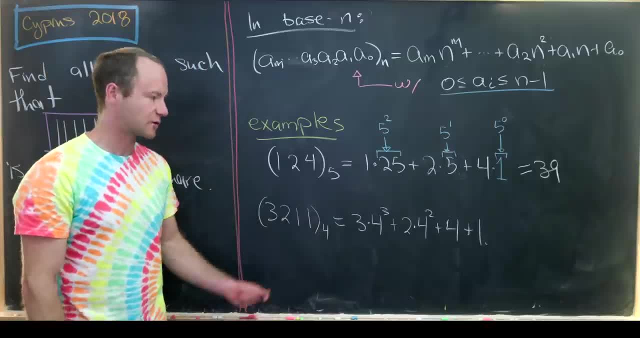 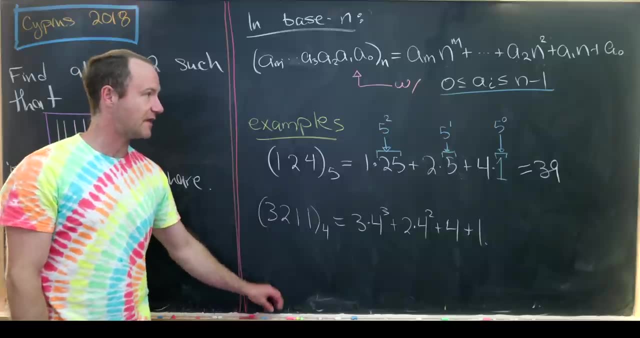 3 times 4 cubed plus 2 times 4 squared, plus 4 plus 1.. so I won't work that out, But you could do a bunch more examples built off of this, Okay, so now that we've got this taken care of, let's jump into our solution. 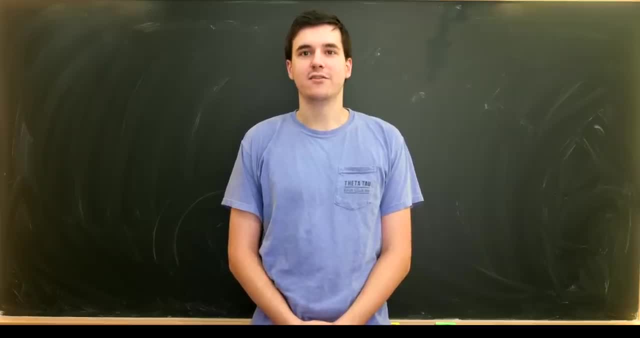 Hey guys, I'm Justin and I'd like to ask you to consider subscribing to the channel. Me and Michael are working really hard towards reaching our goal of Pi 100,000 subscribers by the end of the year, and I believe that we can do it. Thanks for all your support and enjoy the video. 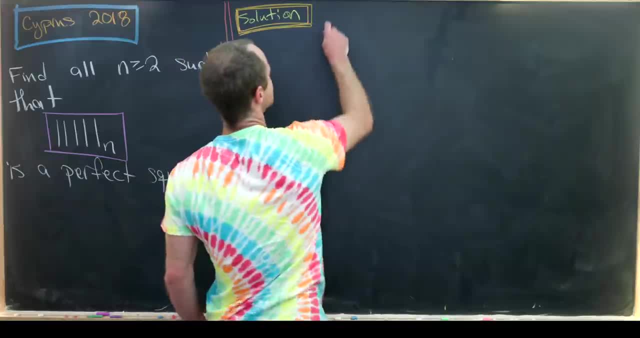 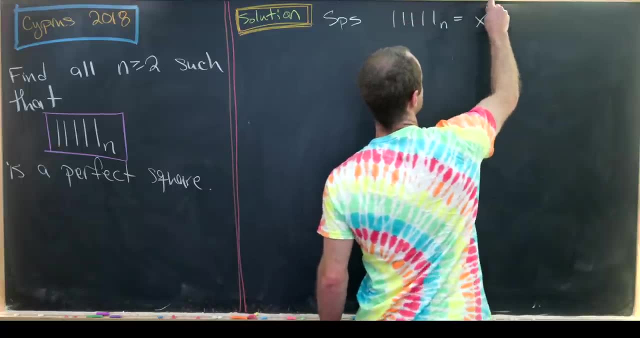 Okay, so now let's go into our solution. So let's start by supposing that 1, 1, 1, 1, 1, so in other words, 5: 1's base n is a perfect square. I'll call that x squared. And now let's. 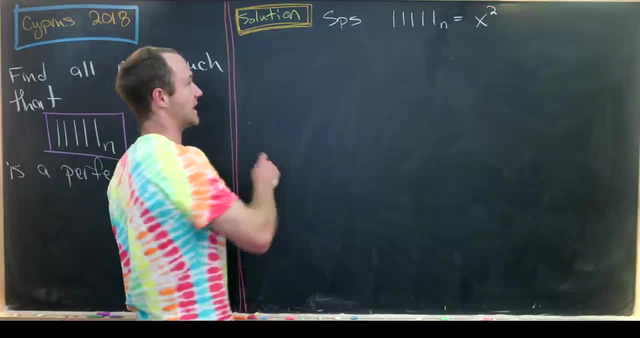 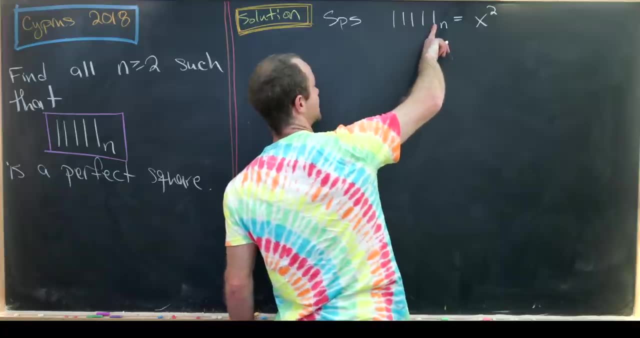 use our formula to write this in kind of a more familiar way. So this is going to be our n to the 0 coefficient. So this is our n to the 0 place, our n to the 1st, 2nd, 3rd, 4th place, and they: 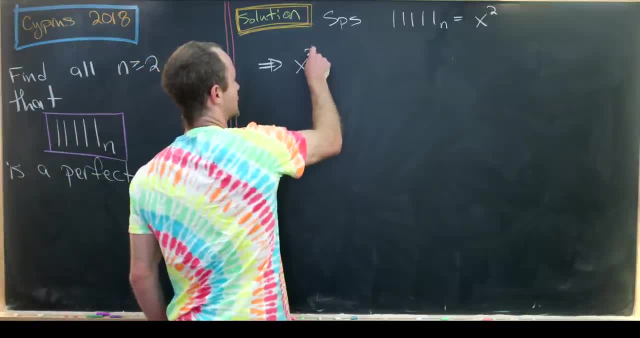 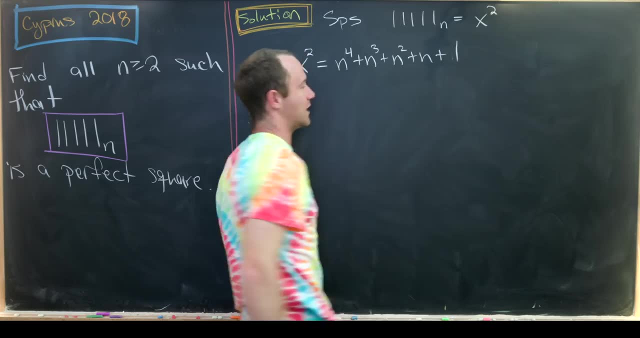 all have a coefficient of 1.. So that means we have the equation x squared equals n to the 4th, plus n cubed plus n squared, squared plus n plus 1.. So in fact this statement over here is equivalent just to finding all. 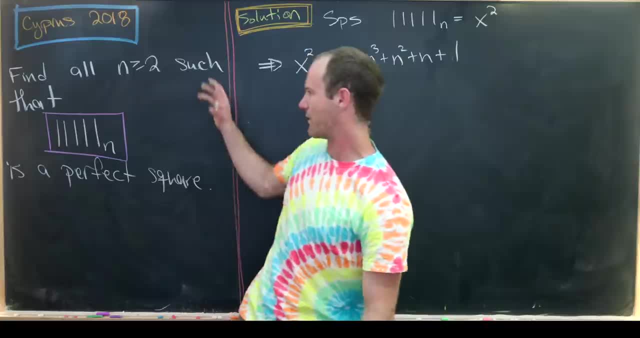 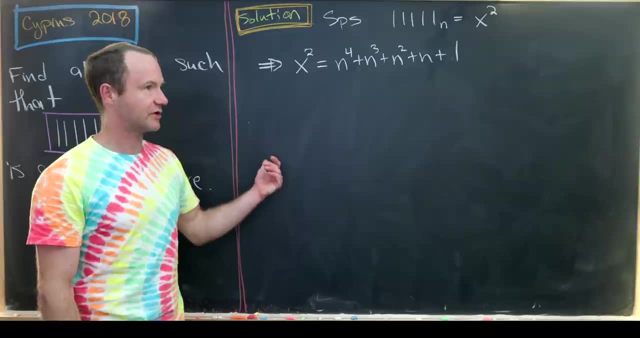 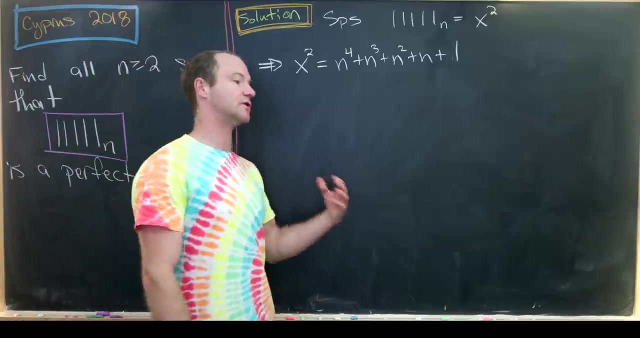 perfect squares of this form, But I think wrapping it up in this statement is like quite a bit nicer. Okay, so now, where could we go from here? Well, generally, when you're asked to find out when things are perfect squares, there's only going to be a few possible small solutions, And also 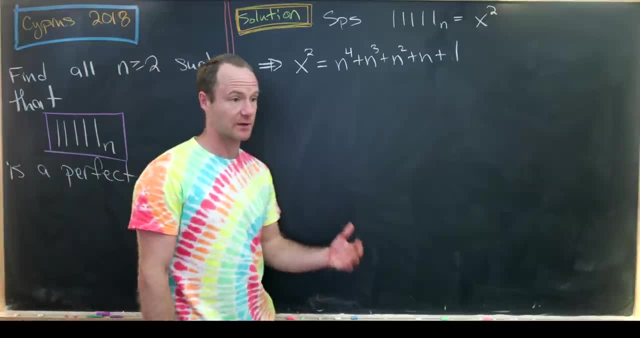 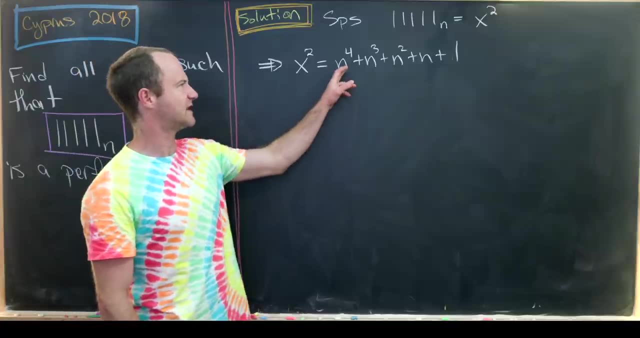 the general strategy for showing something is not a perfect square is to bound it between two consecutive perfect squares. But it turns out that this n to the 4th plus n cubed plus blah, blah, blah term is a little bit hard to deal with. 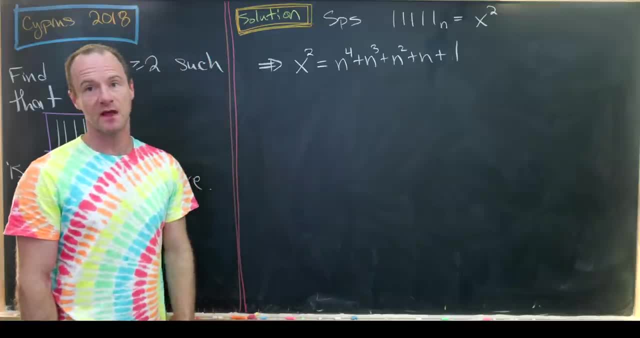 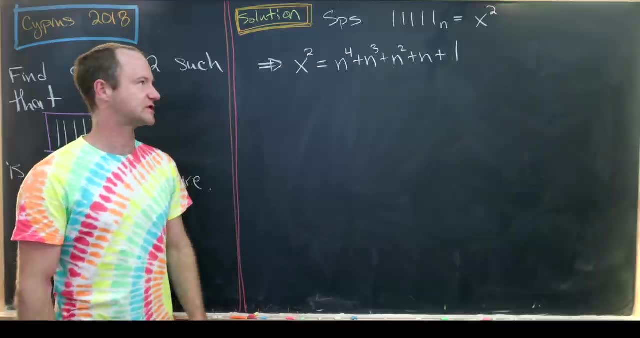 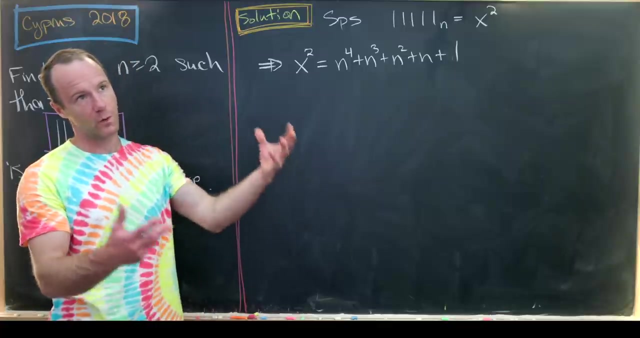 because all the coefficients of these are the same and they're all equal to 1. And whenever you square a binomial or a trinomial, you get different coefficients of these things, Except for the case when the coefficients are 4, then a lot of the coefficients from what you square. 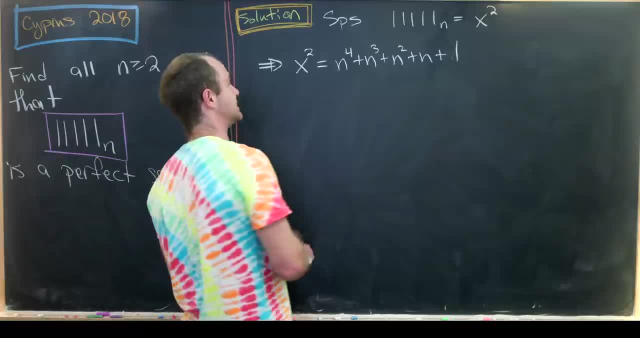 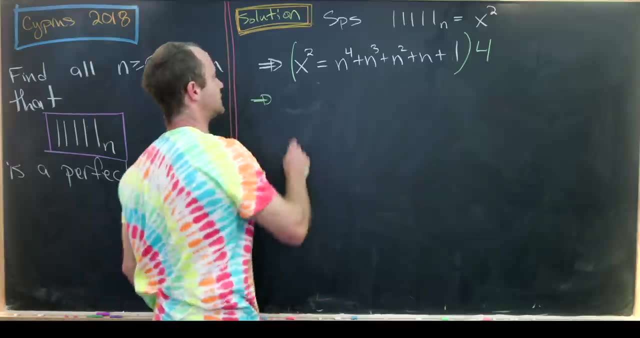 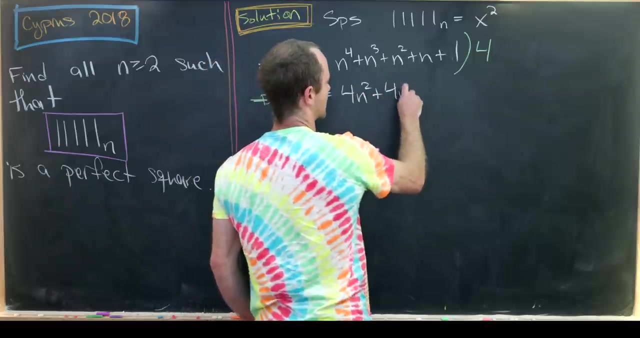 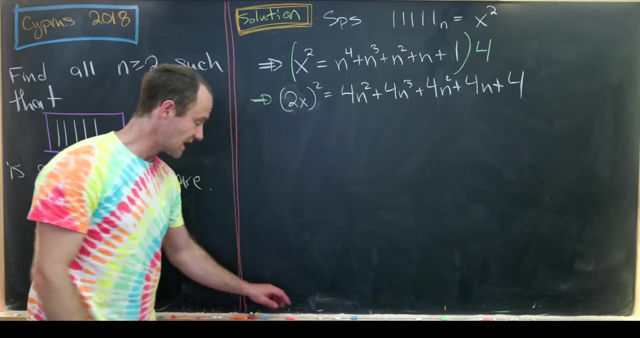 happen to be the same. Anyway, all of this is to be said that this actually motivates us to multiply this whole thing by 4.. And let's notice that'll give us 2x quantity squared equals 4n squared plus 4n cubed, plus 4n squared plus 4n plus 4.. And now our goal is to put this object between: 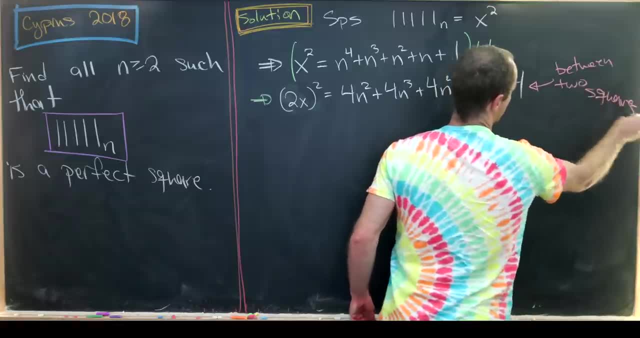 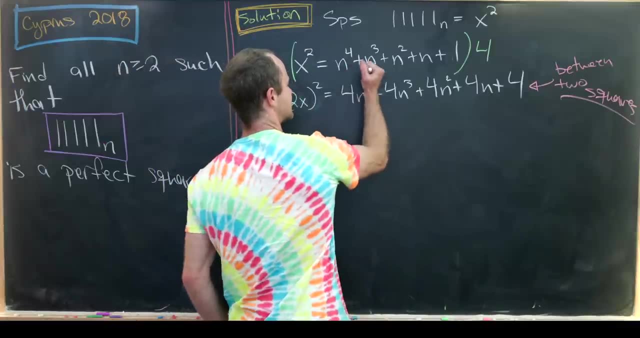 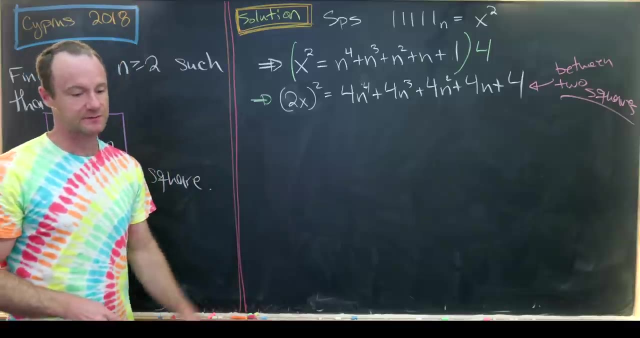 2 squares, Great. So let's maybe see how we could do that. So let's look at the top half of this- And I just noticed this should have been an n to the fourth- And see if we can get a perfect square that mimics the top half of this, And we can, and that'll be 2n squared. 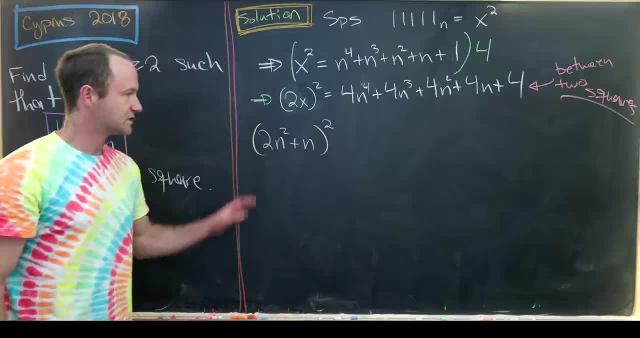 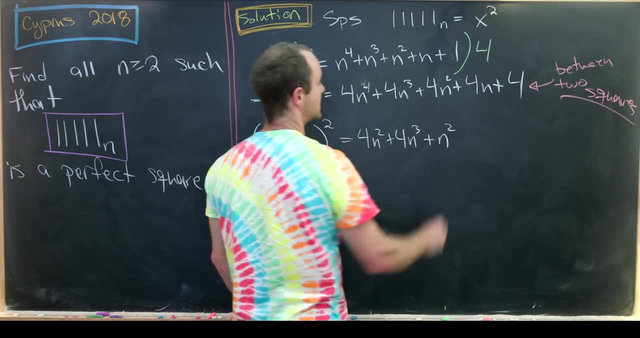 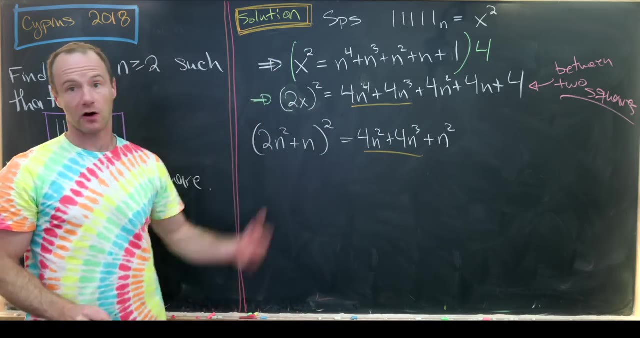 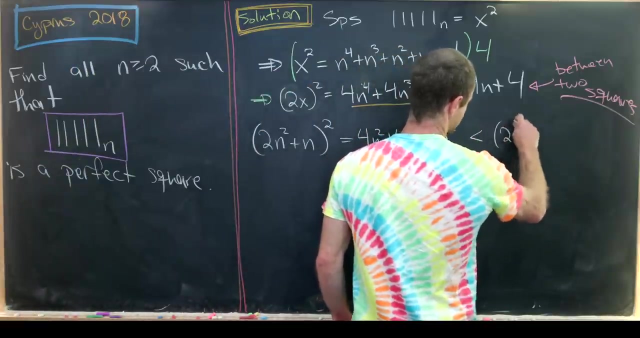 plus n quantity squared. So notice, if we multiply this out, we'll get 4n squared plus plus 4n cubed plus n squared, So that mimics the first two terms of our would-be perfect square. Furthermore, this is very clearly always less than our perfect square. 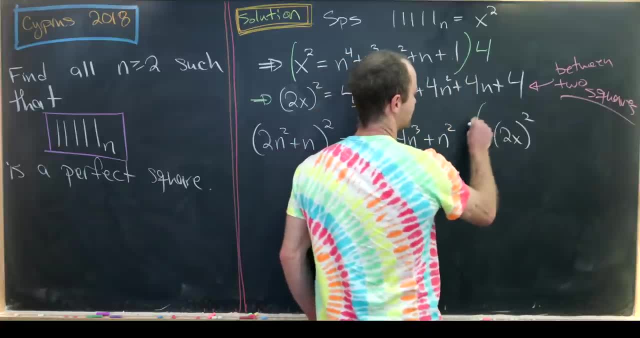 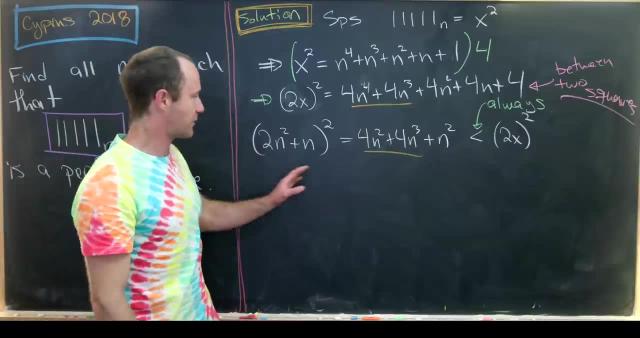 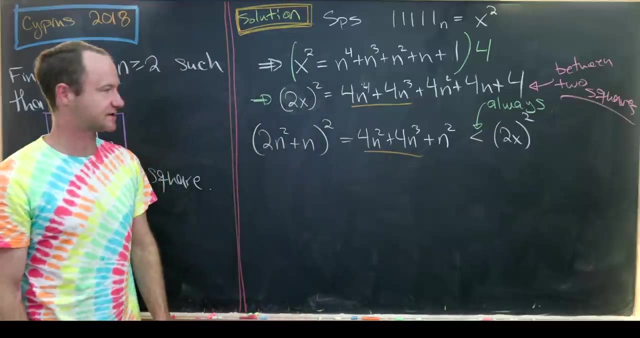 which is 2x squared, And let's just point out that this occurs always. Now, what we'd like to do is hopefully have the perfect square just above this. one is oftentimes larger than 2x squared. Okay, so let's see how we could do that. 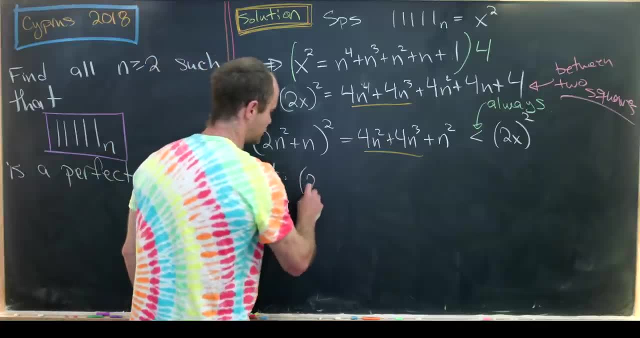 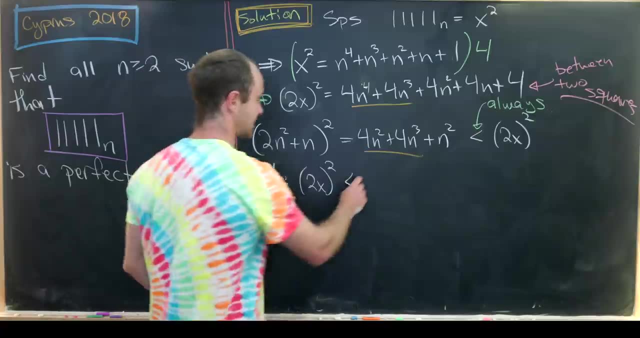 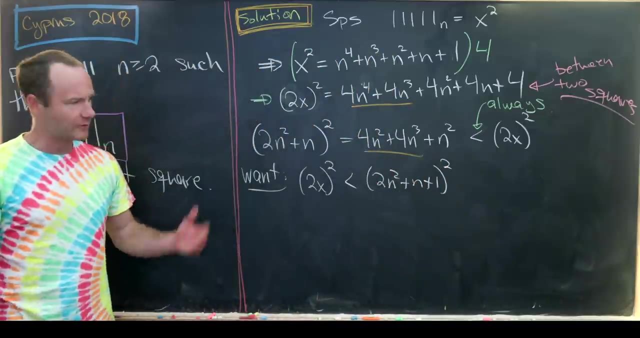 So let's say we want 2x quantity squared, In other words, our object right here to be strictly less than 2n squared plus n plus 1.. 1 quantity squared. So why would that be helpful? Well then, we'll have our perfect square between two consecutive perfect squares. 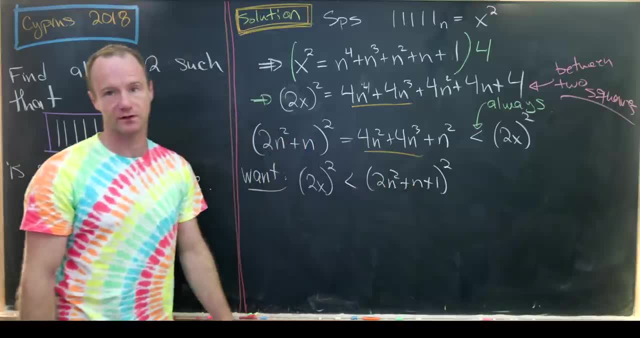 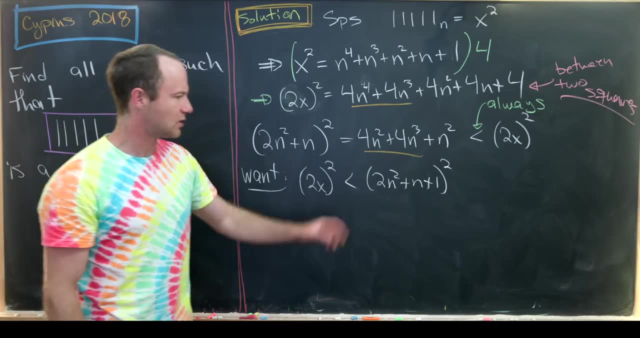 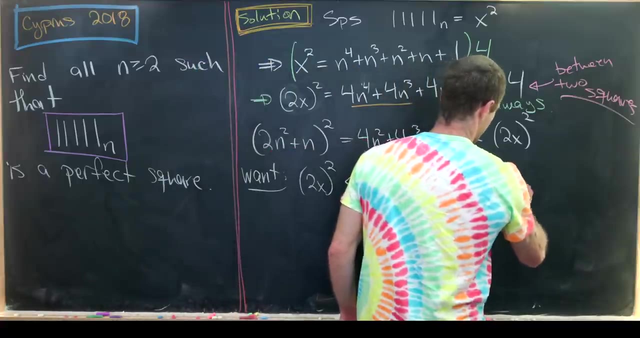 We've got something squared and then that's something plus 1 squared, But clearly there are no perfect squares between two consecutive perfect squares. Okay, so let's maybe multiply this out and see what that really gives us. Multiplying this thing out will give us 4n to the fourth, plus 4n cubed. 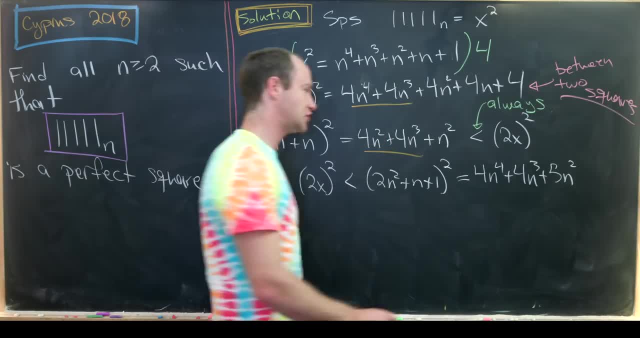 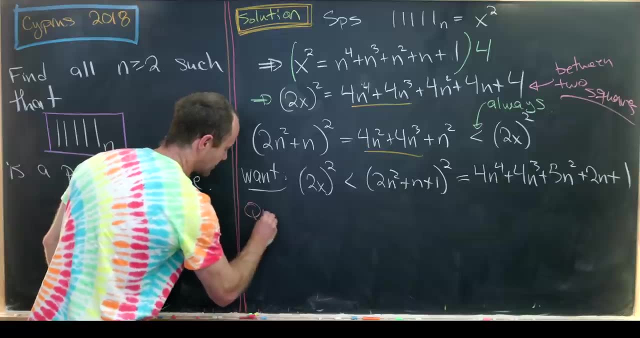 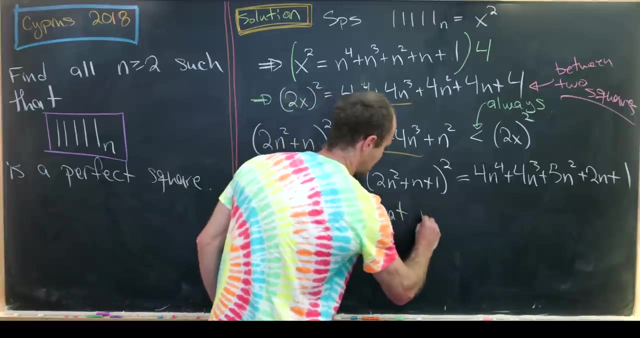 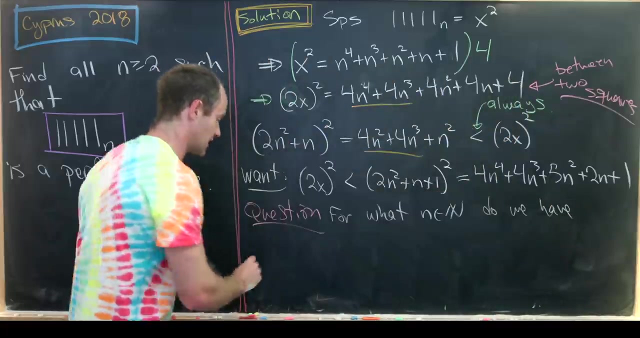 plus 5n squared plus 2n plus 1.. Okay, great, And that motivates the following question. And that will be for what? n? I'll just say natural numbers. do we have this guy right here, which is 4n to the fourth plus 4n cubed? 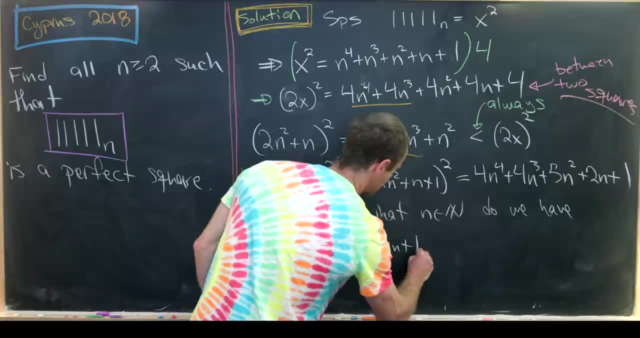 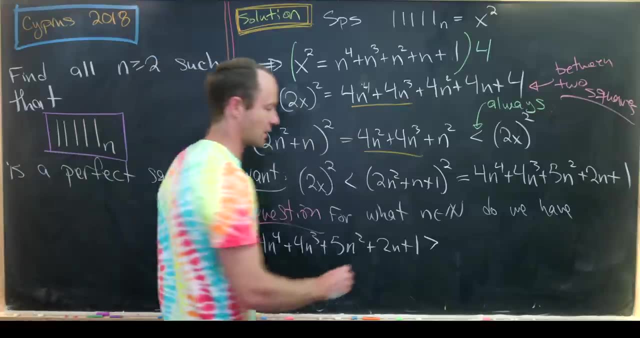 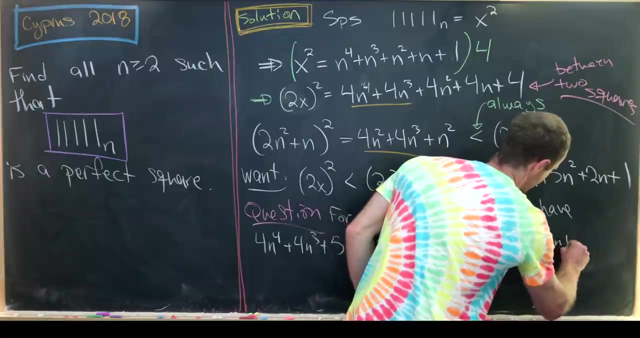 Plus 5n squared plus 2n plus 1 is strictly bigger than this 2x quantity squared. But let's recall this 2x quantity squared was this: 4n to the fourth plus 4n cubed plus 4n squared plus 4n plus 4.. 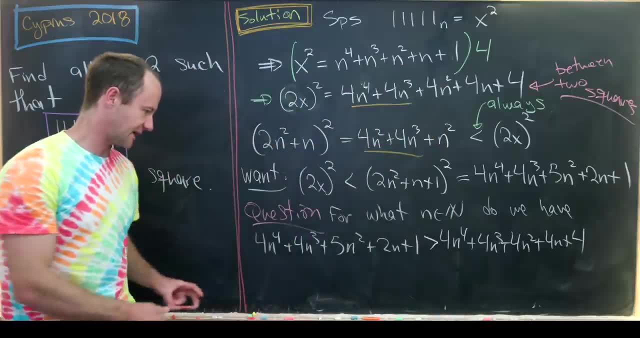 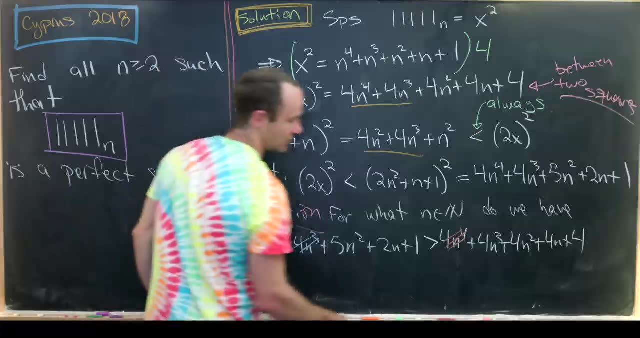 Great, But there's actually quite a bit that can cancel here. This 4n to the fourth will cancel this 4n to the fourth. This 4n cubed. This 4n to the fourth will cancel this 4n to the fourth. 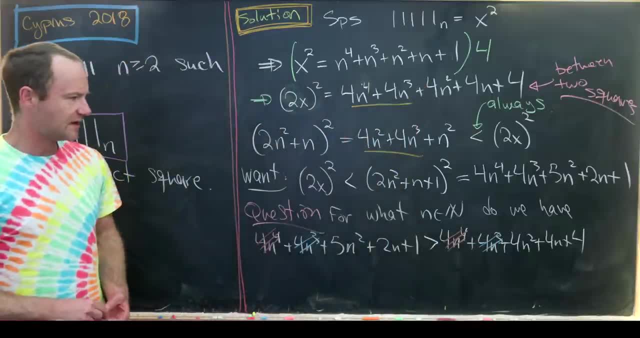 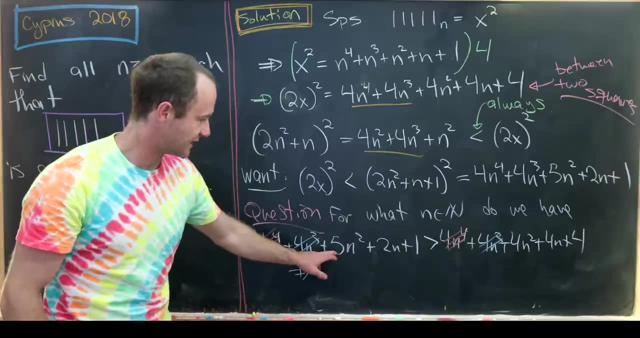 This 4n cubed will cancel this 4n cubed And then we're left with a quadratic inequality. So let's move some things around on that quadratic inequality And notice we get 5n squared minus 4n squared. 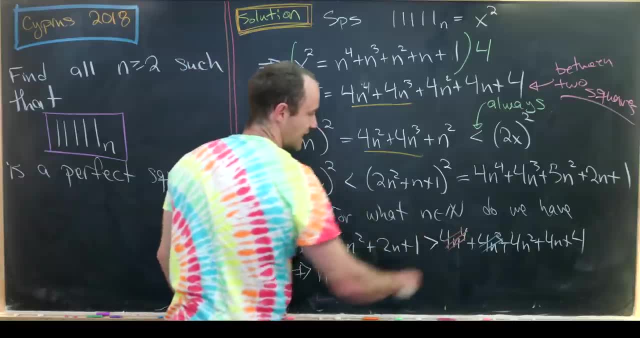 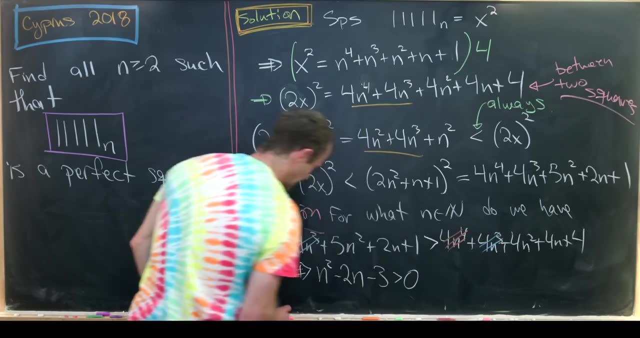 That's going to give us n squared. We have 2n minus 4n. That's going to be minus 2n. And then we have 1 minus 4.. That's going to be minus 3.. So, in other words, we want to determine for what n natural numbers. 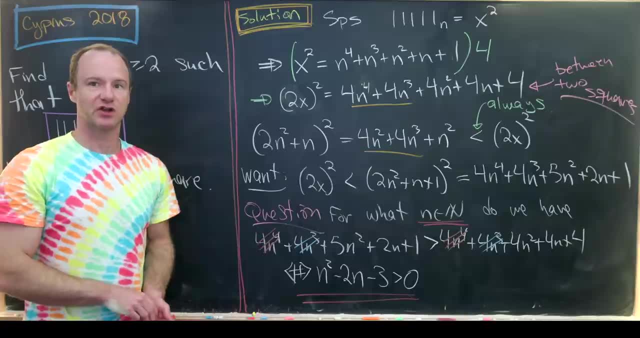 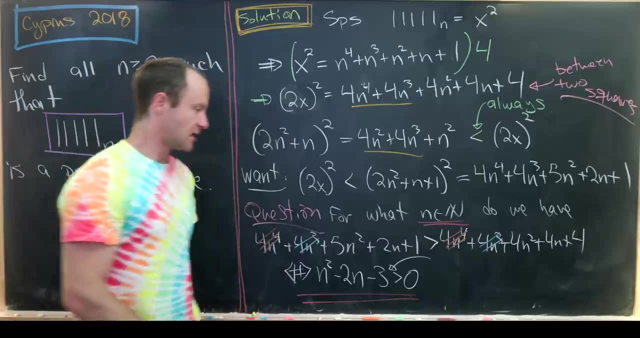 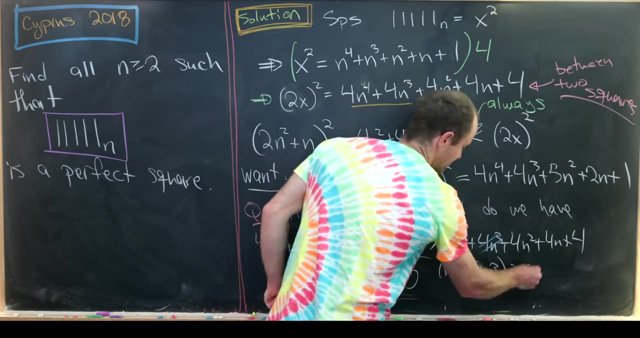 do we have this occurring? This quadratic expression is bigger than 0.. But luckily this quadratic expression is very factorable. We can factor this as n minus 1 times n minus 3. And we want that to be bigger than 0.. 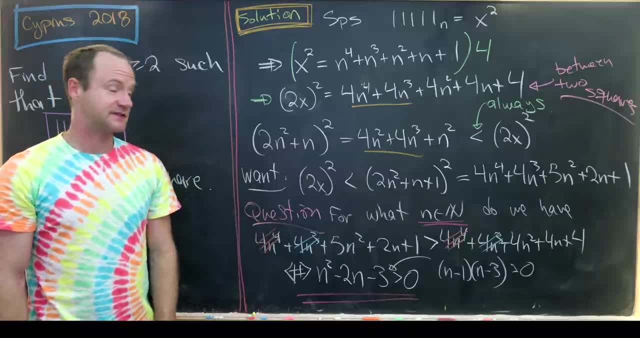 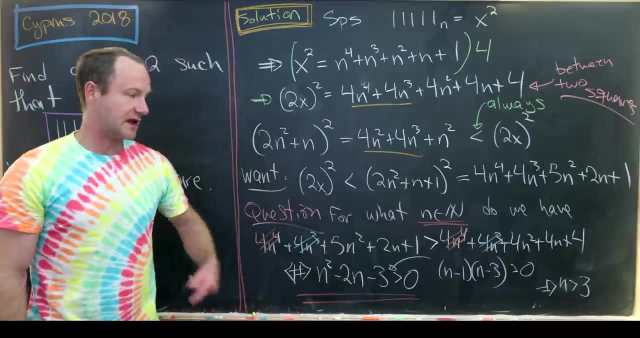 Well notice, that's going to be bigger than 0 when n is bigger than 3.. So here we get, that n is bigger than 3.. Because if n is bigger, If n is bigger than 3, then n minus 3 is bigger than 0 and n minus 1 is bigger than 0. 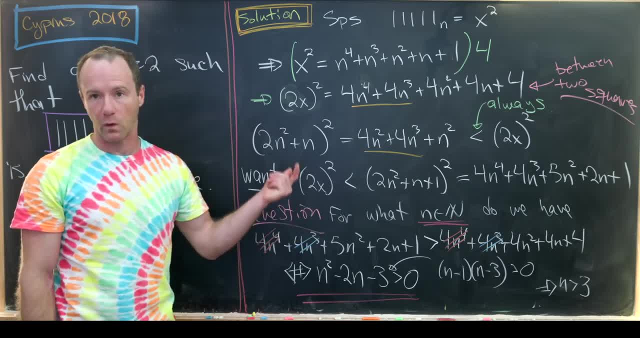 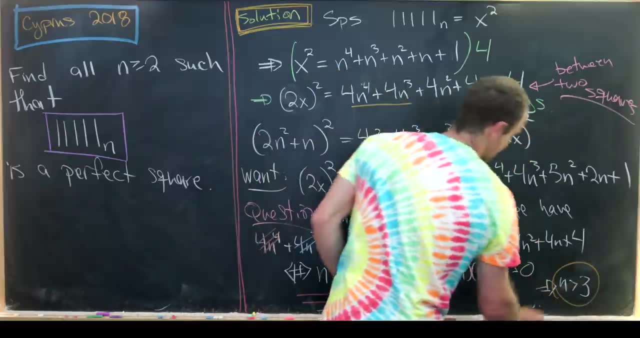 And then, furthermore, the only roots of this polynomial occur at 1 and 3.. And so if you're to the right of 3, you'll always be bigger than 0. So that means we get down here that n is bigger than 3.. 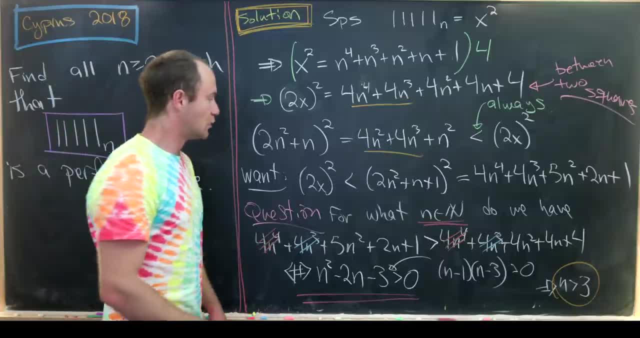 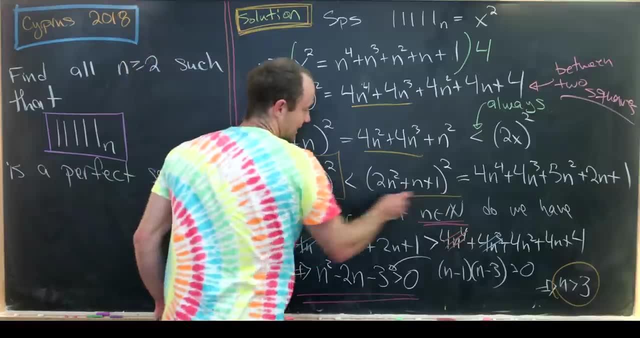 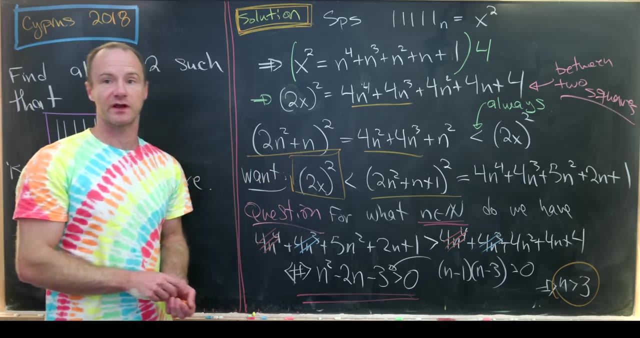 So let's summarize what we've just shown. So we've just shown that our perfect square, this 2x quantity squared, is strictly less than 3.. And strictly bigger than this guy when n is bigger than 3.. Which tells us the only possibilities are for n to be equal to 2 or equal to 3..